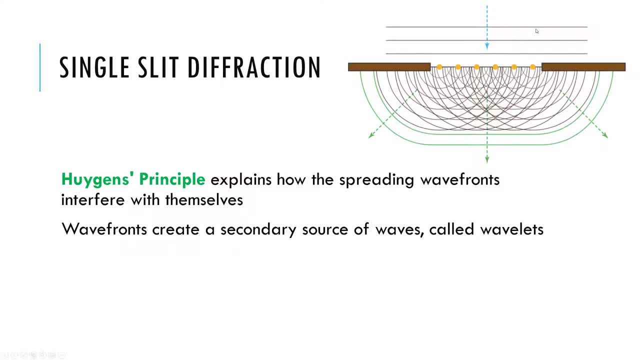 out and see if you could convince yourself that a line of these little dots, all creating circular wave fronts, would connect to make their wavefronts would all overlap and create a straight line in front of them. And then again and again, and again, if I kind of draw and combine, 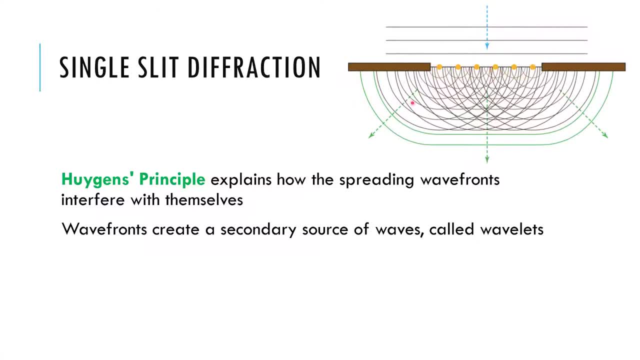 these, I can see that next straight wavefront. This principle is pretty crazy but I'm going to. but it does describe two things. number one: it describes why this kind of diffraction happens like this. because, um, with all of this space there's um, we get. the next line is a straight line. 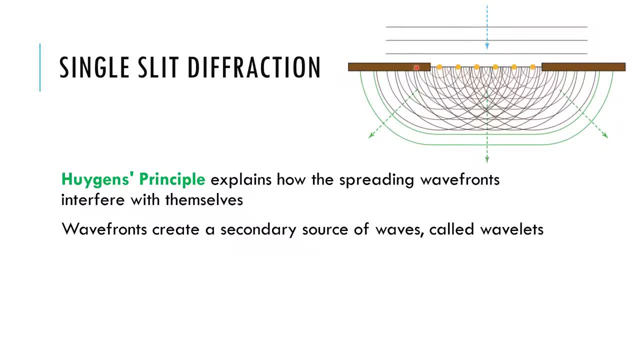 but when they come through the opening there's no more wavelets over here. so the wave fronts created by this little wave wavelet uh do kind of bend. we get the bendiness from the sides here and that's why we kind of get. you know, the diffracted wave front is sort of flatter in the middle. 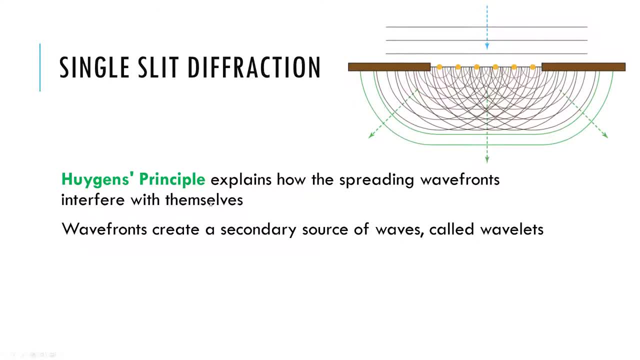 but it is rounded off on the edges right. that kind of explains this and it also explains this interference. the idea is that the waves, individual little waves from these wavelets can interfere with one another. so that's what we're looking for: the math of single slit. 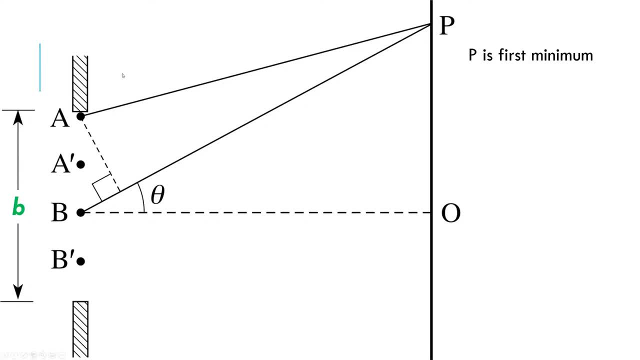 okay. so here's the concept, here's the setup, here's how this equation is derived. again, you get this equation in your data booklet, but this is another one where it is useful to know the derivation, where it comes from, understand the geometry happening. uh, especially okay. so a, a, prime, b, b, prime, all represent wavelets, the main concept. 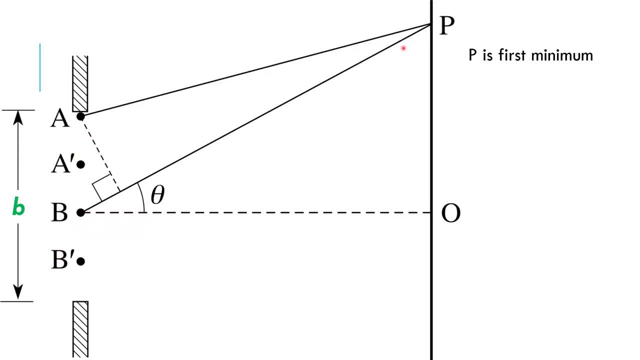 is this: this is another kind of tricky one, but what we want to focus on is the minimum, the first minimum, because that's where destructive interference, hap, is happening. so that's probably one of the um most straightforward places to look to come up with some math and the idea is here. 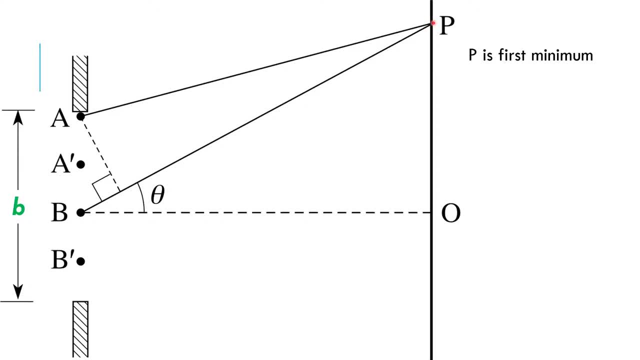 all of the wavelets must be canceling each other out. there's total destructive interference here, because i do get a dark spot if there's like an infinite number of wavelets, whoa, we got to think about how we could get all of them canceling out. uh, here's the kind of trick. 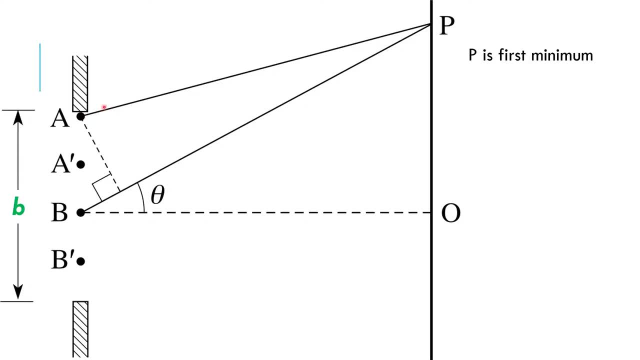 uh, the setup here is that every wavelet interferes with another wavelet exactly halfway down the slit. so here's wavelet a right, at the very, very, very top of the slit, and here's wavelet b right, smack in the middle. these two are interfering with one another destructively. 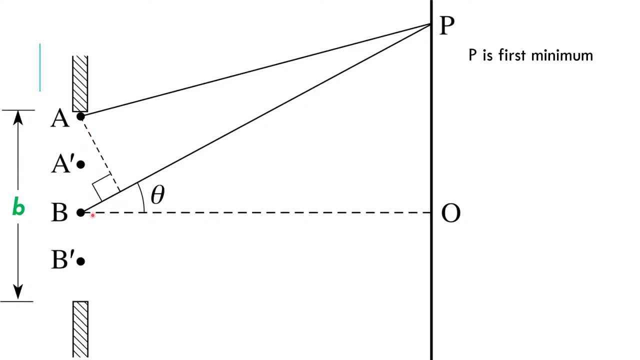 if that's the case, then every wavelet will have a buddy halfway down the slit that it interferes with. so, for example, a prime- maybe a quarter of the way down- is going to interfere with b prime, maybe three quarters of the way down, and they'll cancel out all right and there. 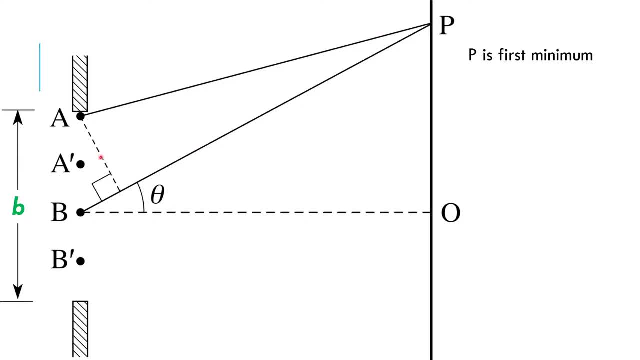 is like an a double prime right here and a b double prime right here and they cancel out. and so if every wavelet has an accompanying wavelet halfway down the slit, then even if there's- quote unquote- infinity of them, they will all cancel out with their partner. 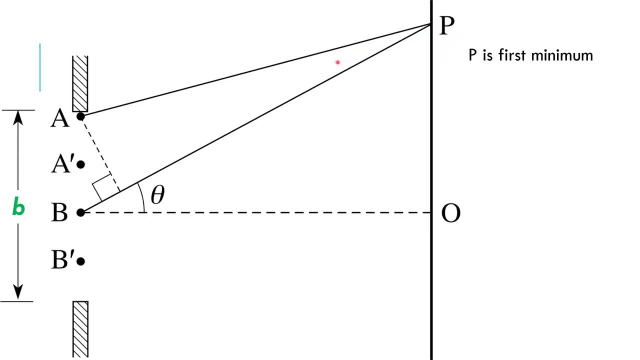 and at p i would get total destructive interference. that's the concept. again, meditate on that a little bit. that's a that's a tricky one, uh, but that's the concept. so we're going to be looking at half of the slit. for that reason, some variables introduce the width of the slit. incident single: 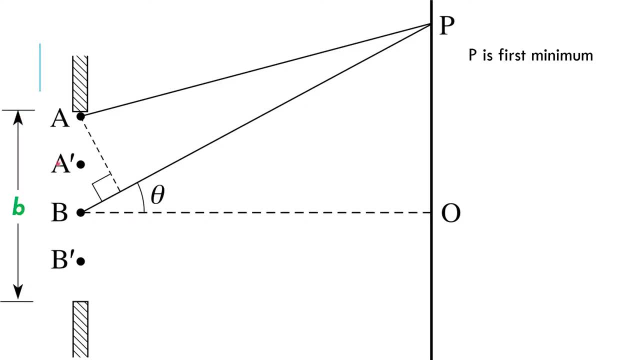 slit interference we call little b. little b is going to be the size of the opening traditionally referred to as the form for a single slit, and so, splicing over that, this will be an opportunity for us to find out what that is going to look like and what we're going to use. 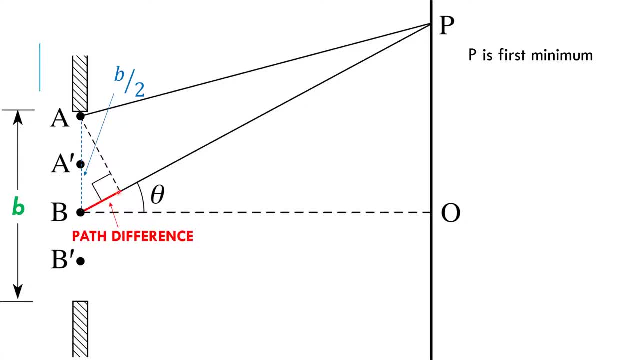 all right. so, of course, when we create our little right triangle here to look at a path difference, we're dealing with a, b over two hypotenuse and this is the path difference. again, just like when we did the double slit, we're making some. or the two source interference, uh, we're making some. 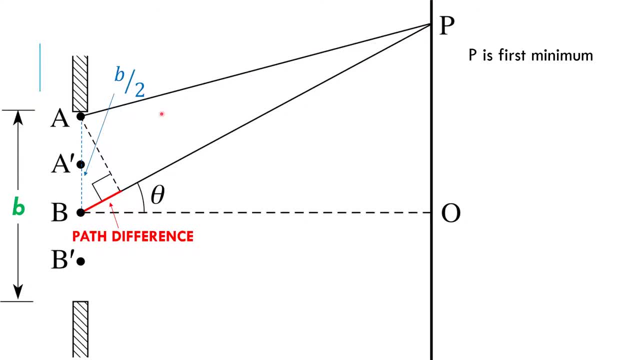 assumptions which, again, the diagram is not nearly to scale, but we are assuming that this line is more or less parallel with this line and for the distances and sizes and such that we'll be working with that in the future, that really is a very good assumption, all right, but that being the case, this is the path difference. 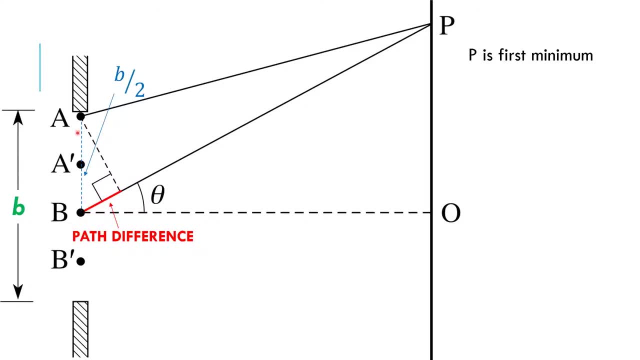 this is how much further the wave from b has to go compared to the wave from a and, of course, for interference, it's all about the path difference. so we got to set this up with path difference, all right, and at the first minimum, the idea is going to be that the path difference uh. 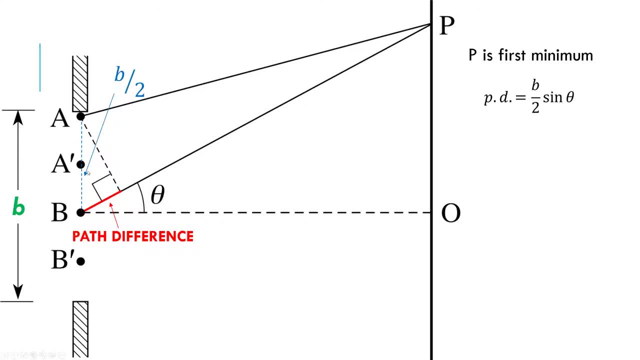 is going to be. we can do some trigonometry here, so we're doing some sohcatoa um and might not be in here. all right, this angle is the same as this angle, just like before, similar right triangles. so i take the sine of that angle. uh, solve for my path. 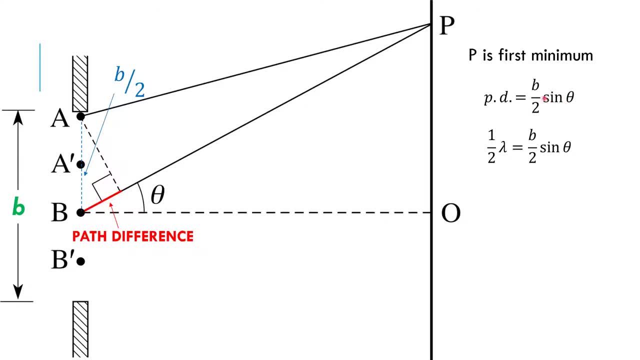 difference, the opposite leg, and i get b over 2, the hypotenuse times the sine of this angle, which is the angle of the wave from a to b. we say to the first minimum like this: all right, and if that's my first minimum, remember how. 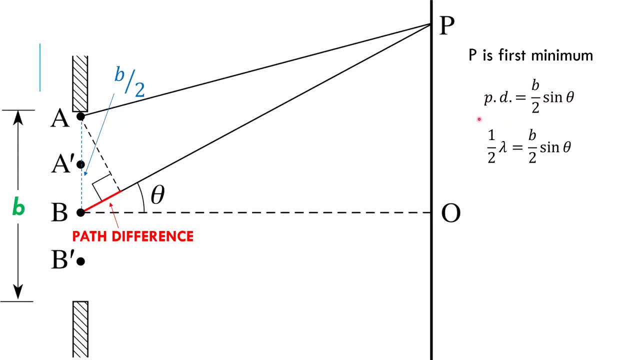 destructive interference works. i get destructive interference when i'm off by a half number of wavelengths. so if the path difference is half a wavelength they're going to cancel out crests and troughs, line up total destructive interference. it could be one and a half wavelengths or two, and 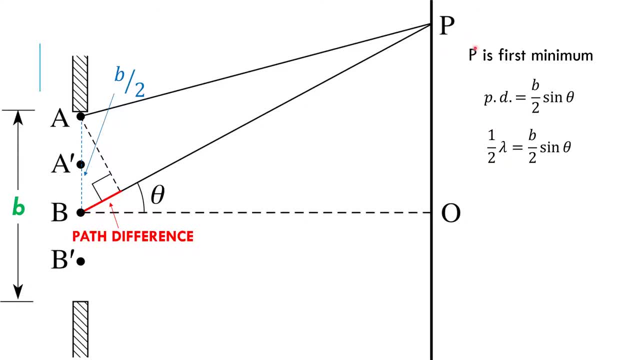 a half wavelengths or nine hundred and a half wavelengths, but since this is my first minimum over here, the path difference is zero. path difference increases and increases, increasing until half a wavelength. that's the first time i'll see the stark spot. so there's the setup: that path difference is half a wavelength. 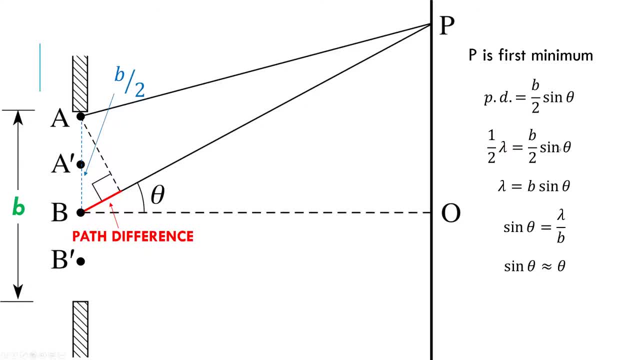 now we math, math, math, math. um, when we solve for the, for the angle is typically uh, what we're going to look at here we're going to get the sine of the angle is equal to the wavelength divided by the size of the slit. and here is another small angle approximation, believe it or not. 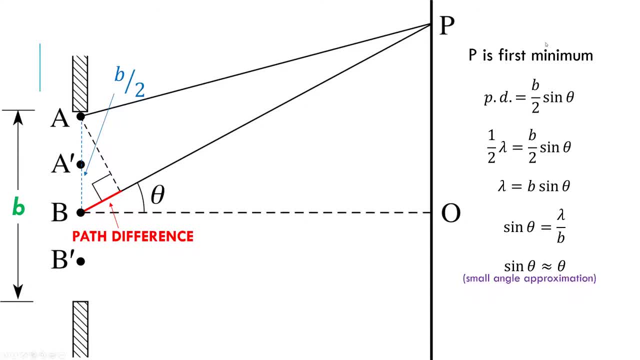 we're going to do this. the sine of theta is: yeah, it's about the same thing as theta. they're basically the same thing. all right. again, this works for small angles only, so usually less than like five degrees. um ten degrees it starts getting a little funky, but still pretty good. 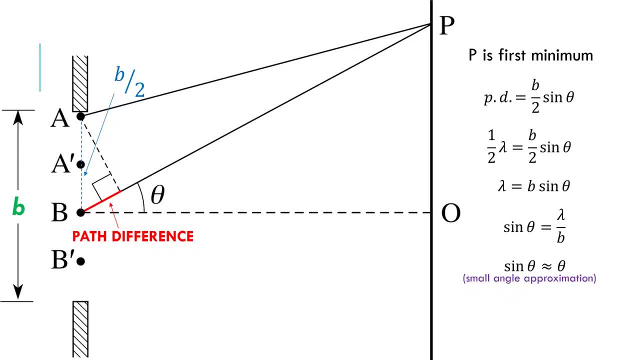 uh, one thing to note here is: you definitely need to be in radians. be in radians, right. so like, try it out. try it out. take the sine of i don't know 0.01 with a sine of 0.05 radians. you'll see that you get some very, very, very close. 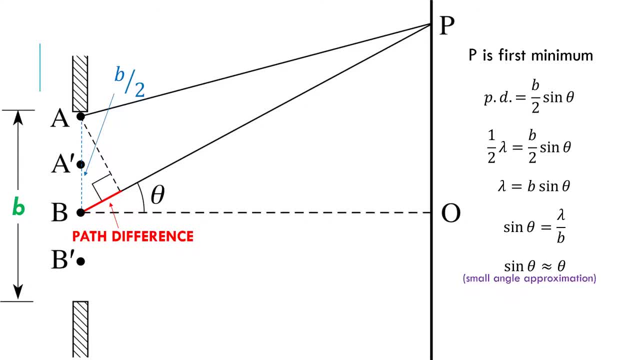 answers when we're dealing with these small angles. all right, remember, we can also say that's more or less the same as the tangent of the angle. all of these things at small angles are very close to each other and certainly we're not going to be doing dealing with enough precision where it's gonna matter, where. 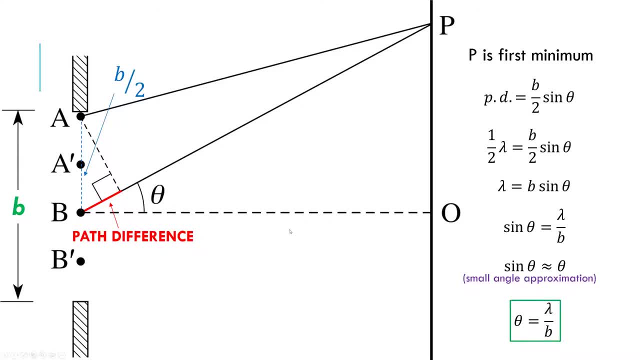 that rounding happens all right. so, all that being said, this single slit equation is this: angle equals wavelength over B. this just shows up in the data booklet under single slit diffraction. so you need to bring some knowledge, like with the whole data booklet, which is mainly what these 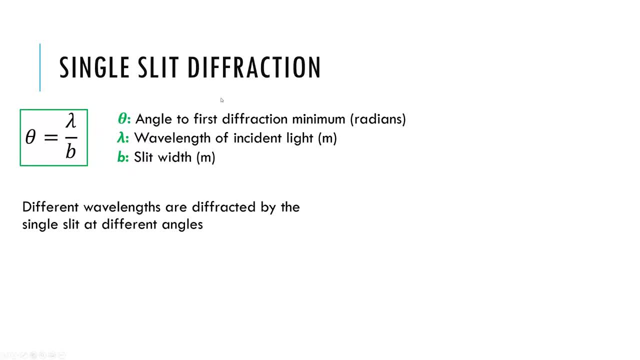 variables are. so it is a very specific angle. it's the angle to the first diffraction minimum and it's got to be in radians since we're using the small angle approximation. that's the angle to the minimum of a single slit diffraction in radians. it's a very specific equation. lambda is, as always, the wavelength of the. 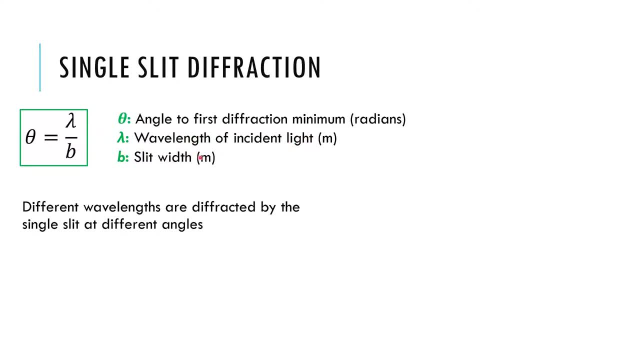 incident, light, the light coming into the slit, and B is the width of the slit, size of the opening. all right, the main thing this equation tells me, one concept that you want to be able to picture and think about here- is that the angle to that dark spot depends on the wavelength. the different 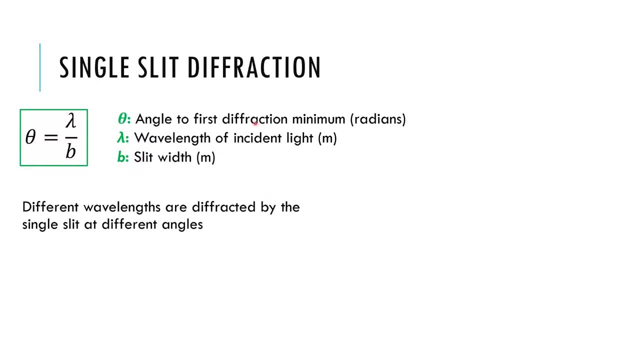 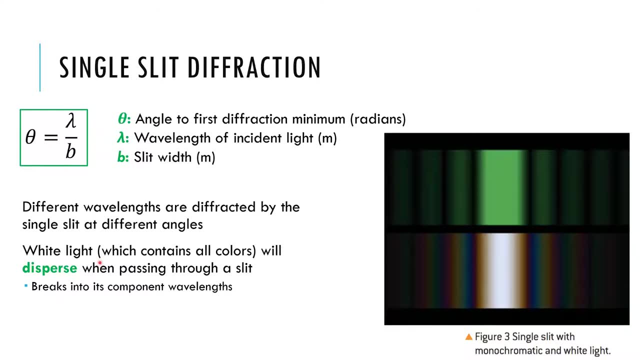 wavelengths will be diffracted at different angles, red light will be spread out a different amount than blue light, and so on. alright, this is one way we can see dispersion of light, which is- remember, white light is all of the colors of light happening together, superimposed on. 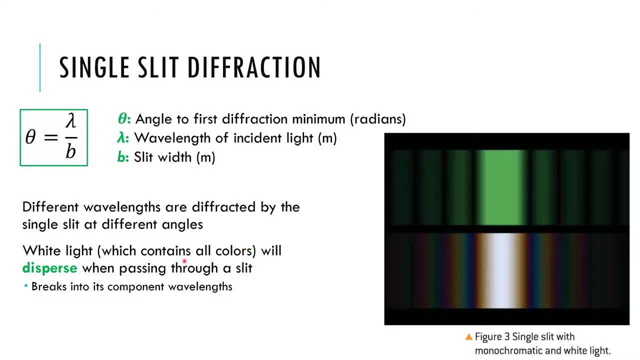 each other in your brain. when it sees that goes: whoa white light. you see red and green and blue and orange and yellow and yadda yadda all together. if I send white light through an opening then the red parts are going to spread by a. 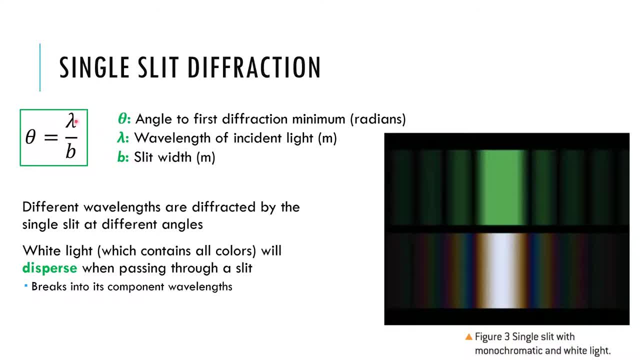 certain angle the blue parts will spread by a distance angle. good exercises, he want to be able to do this. think about which one will get spread more versus less, and why. all right. but you can see here you get this, this fringing and this almost rainbow effect. you can see the red light and the 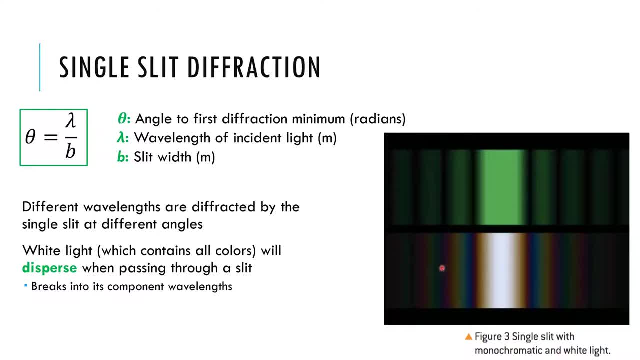 blue light being split and separated by different amounts, and you get this rainbow fringing especially out at further maxima. all right, so it breaks light up into its component wavelengths, it splits the red differently than the blue and everything in between, and so we can take that white light and we call. 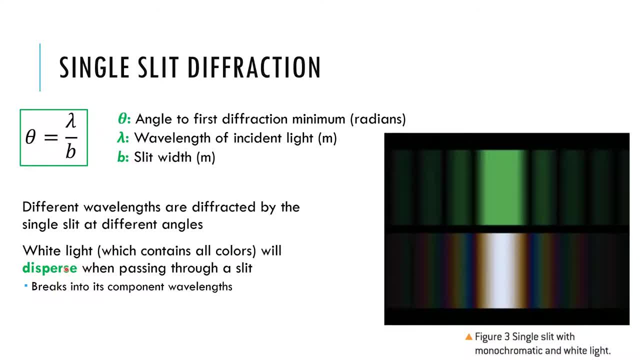 that dispersion whenever you're breaking light up into its component pieces. this is one way to do it. there are other ways, like with prisms and some other ideas- but that the single slit will disperse light for that reason. so that concept, this relationship you want to be able to talk about. 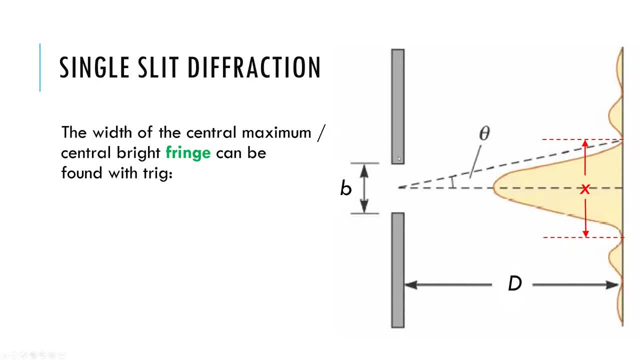 okay, last kind of thing that the IB likes to ask you to do. it's pretty common. you know the angle is not necessarily easy to do, but it's pretty common to do. it's pretty common to do. it's pretty easy to do. it's pretty common to do. it's pretty common to do. it's pretty. 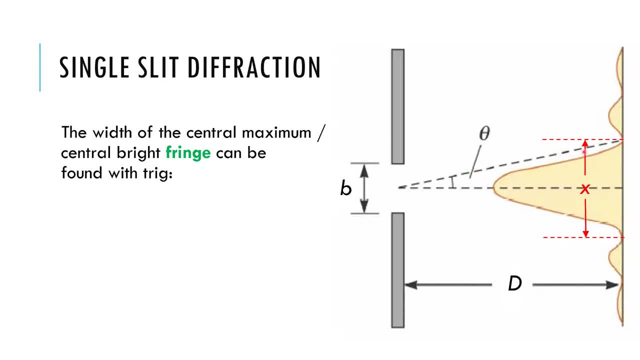 easy to measure. you can imagine, because you have this pattern on a wall. what's? very easy to measure those: how wide the bright spot is. you can get a ruler and just measure it. so the width of the central bright fringe- we call these fringes a lot, these bright and dark spots, the width- here we can use some. 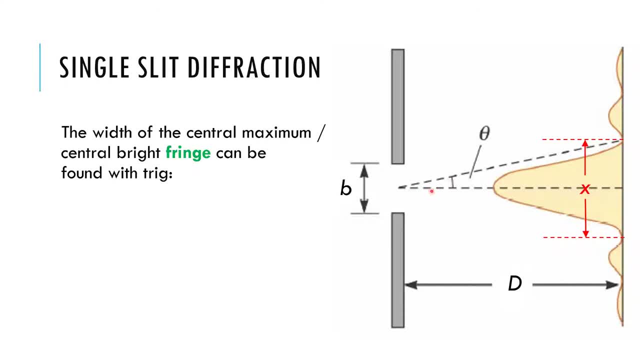 trig and solve. all right. there's the angle to the minimum. remember, it's the angle to the minimum. there's X, so let's see how do we want to set this up? let's do some more small angle approximation. How do you like that? All right, If I take the tangent of, 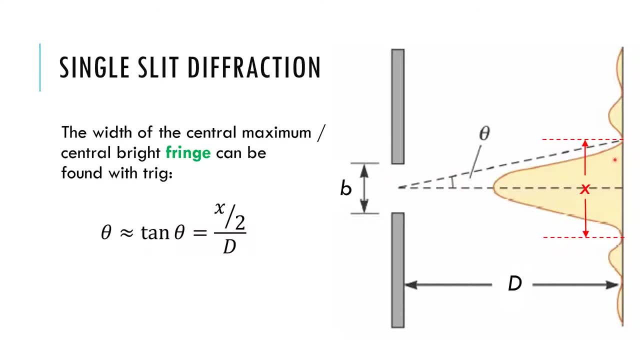 this angle it will be equal to half of the width divided by the distance to the screen. That's opposite over adjacent, All right, And so I can solve for the width of the- sorry, the width of this bright spot, just by substitute, again solving for X here, And so the width of that bright spot. 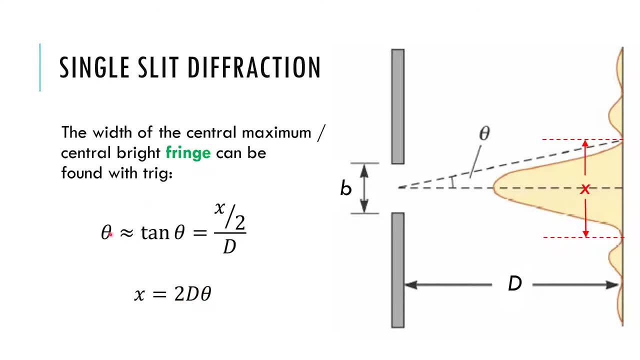 should be twice the distance to the screen times, the angle in radians, because that's about the same as the tangent of the angle. All right, That can give you the width. You definitely want to be able to know how to do this. You can sketch the triangle quickly to you know. figure out that. 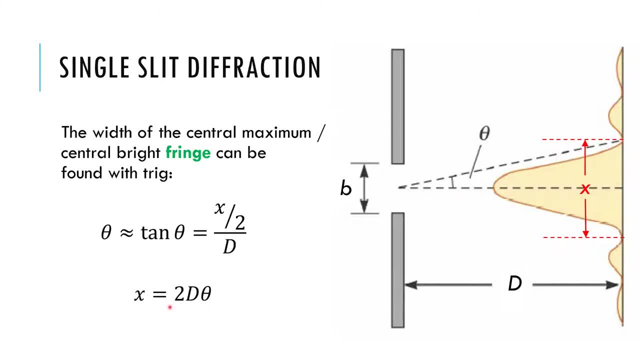 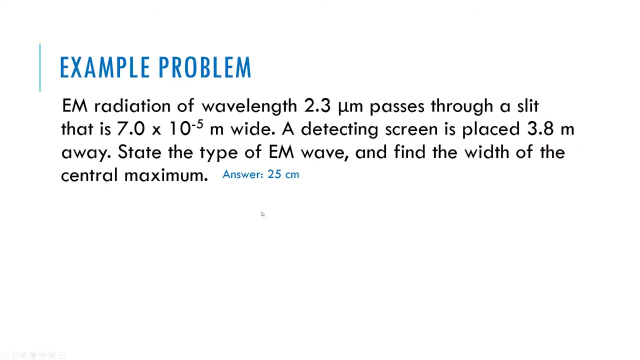 width. So it's all right. triangles that you want to be able to think about, All right. With that being said, here is a problem. You give it a shot, Try it out, See if you can use that, see if you can use that equation and just walk through those. 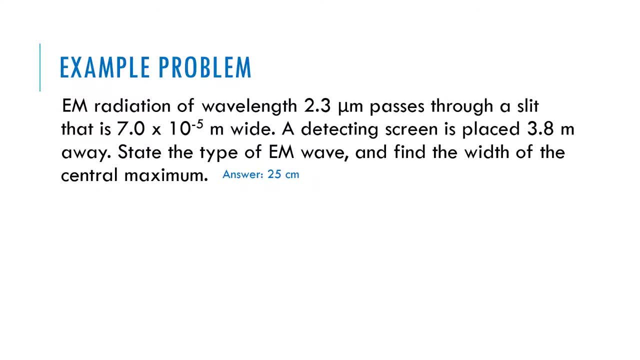 This is a pretty straightforward application of those equations, but this is exactly the type of thing that the IB might ask you to do. So go ahead, pause the video, give it a shot. The answer is there so you can see if you're on the right track. but I'll show you a kind of worked out quick. 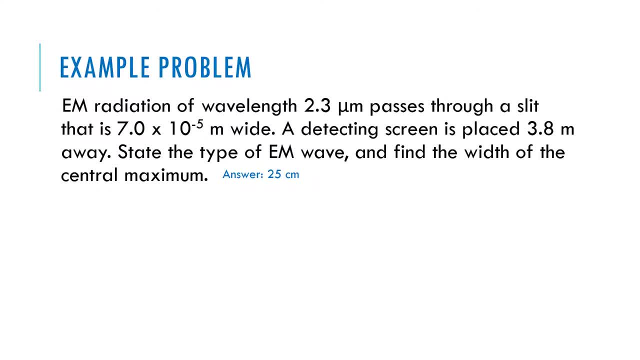 solution in three seconds. Hey, you're back. Okay, Here it is. We're going to use, of course, the single slit equation. Now we're going to use the wavelength of light, Of course. just be careful with your units. I have 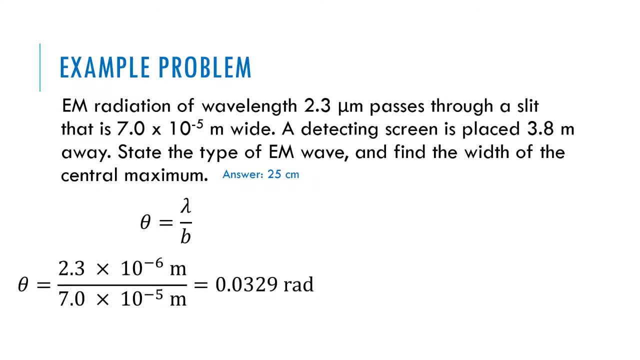 micrometers, which is a pretty common type of thing to see for the wavelength of some kind of light. And so there we go. We're going to convert that to 10, to the minus six is what micro means. We're going to divide by the width of the slit. and there's my angle in radian. So that's the. 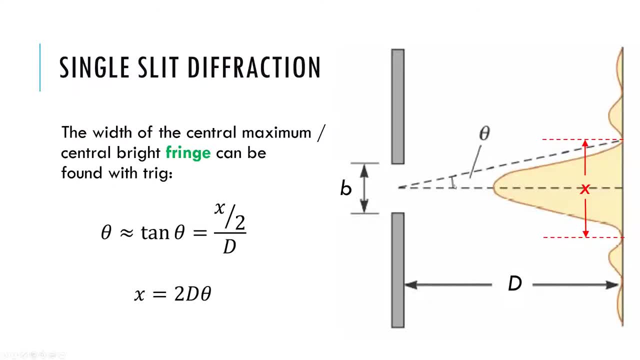 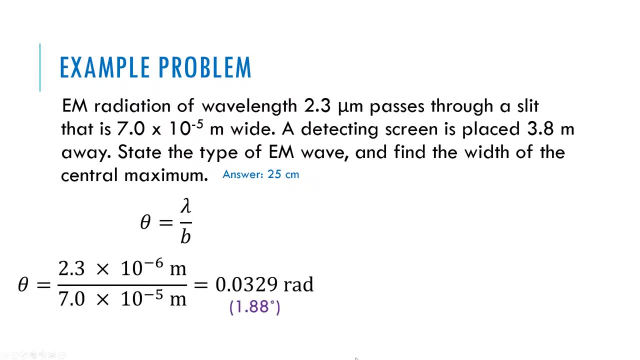 angle, Remember, to the first minimum. that's this angle here, right there, Just for reference. that's about one second. So we're going to use the wavelength of light, 1.88 degrees. If you need to be convinced that we totally are okay using small angle. 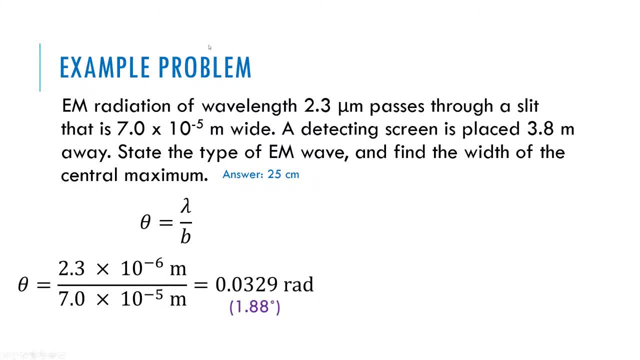 approximation. If you still don't believe me, go for it, Try it. Put the sine of 0.0329 radians into your calculator in radian mode and put the tangent of 0.0329 radians into your calculator in radian mode. I bet you get about the same decimal for all those answers. All right, So for 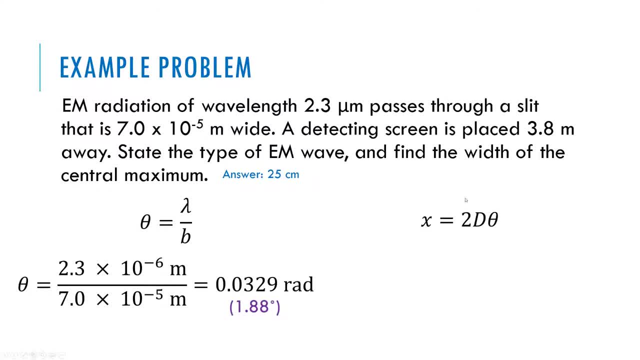 that reason we're going to use our small angle approximation again over here. Multiply two by the distance to the screen, Multiply two by that angle, Simple, simple, And I get it's about 25 centimeters wide, All right So. 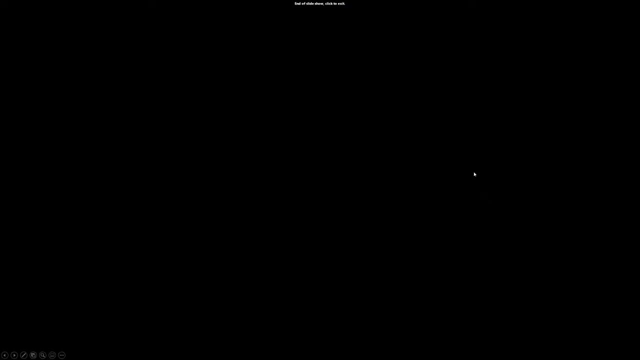 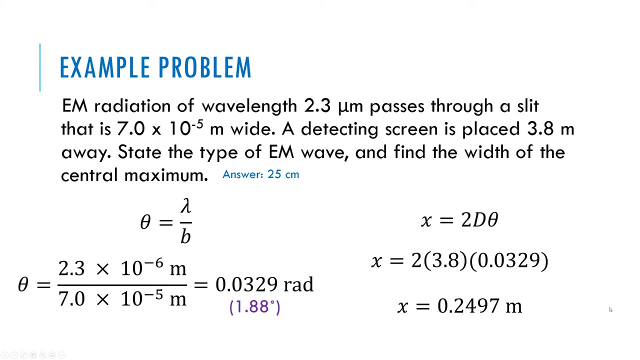 there you go. That's the equation, That's how you use it. There is plenty of fun to be had with single slit diffraction, but those are the basics so that you can go cut loose All right, Have fun.